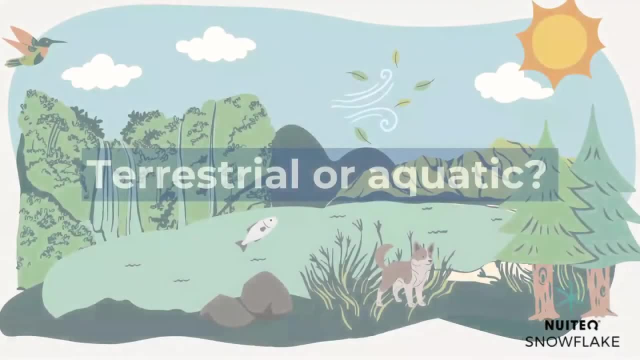 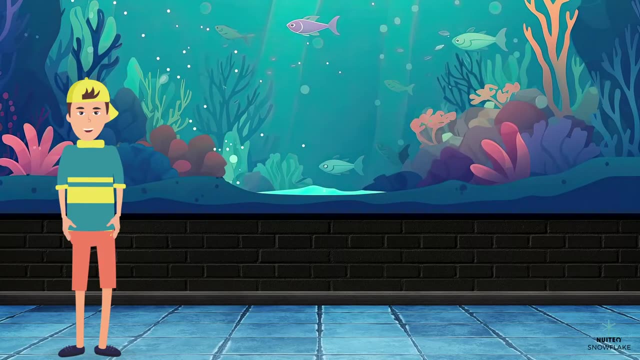 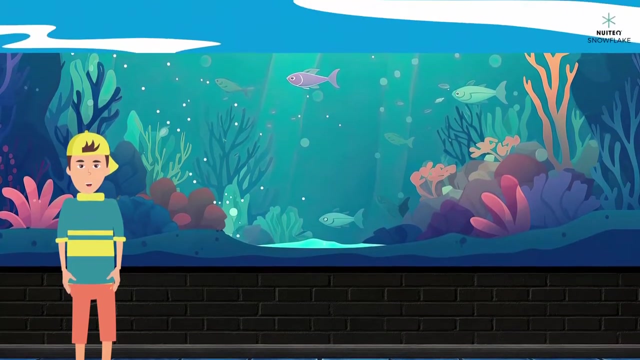 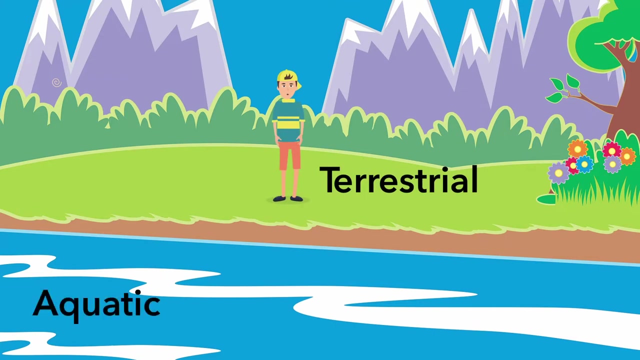 Hi there. Today, we're going to learn about two types of animals: Terrestrial, aquatic animals. Habitat is a fancy word, that means where an animal lives. Terrestrial animals live on land, like you and me. Aquatic animals, on the other hand, live in water, like fish, dolphins and whales. 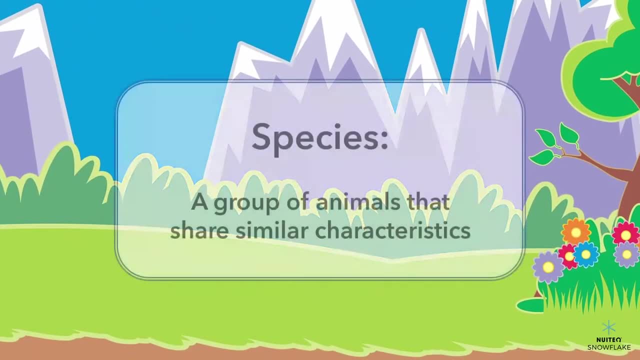 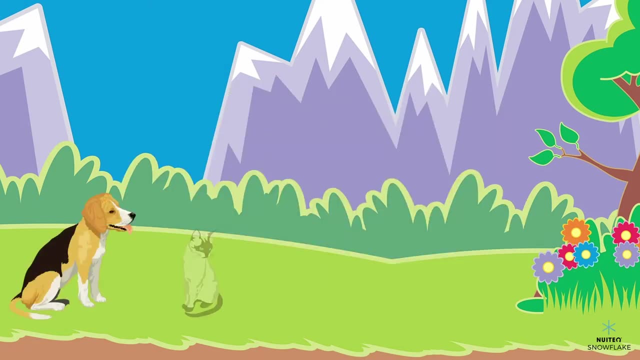 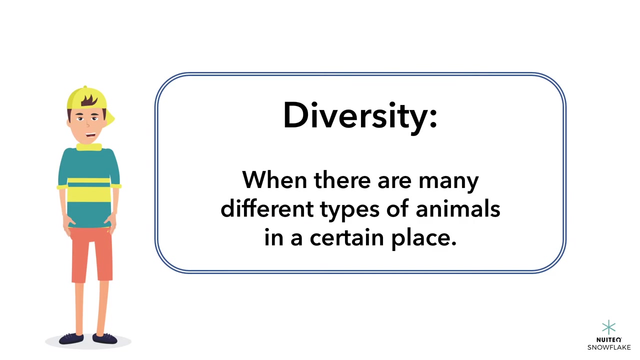 Species is another big word. that means a group of animals that share similar characteristics. For example, dogs, cats and lions are all different species because they have different traits like fur, teeth and claws. Now let's talk about diversity. Diversity means that there are many different types of animals in a certain place. 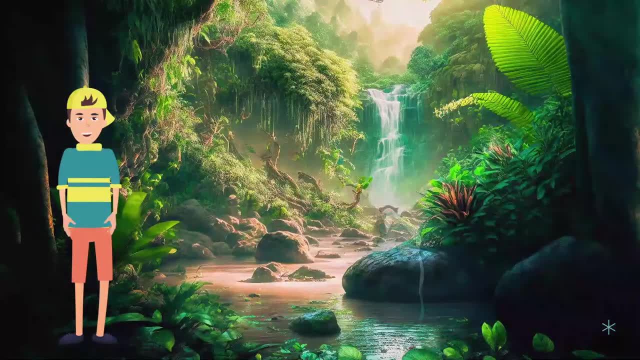 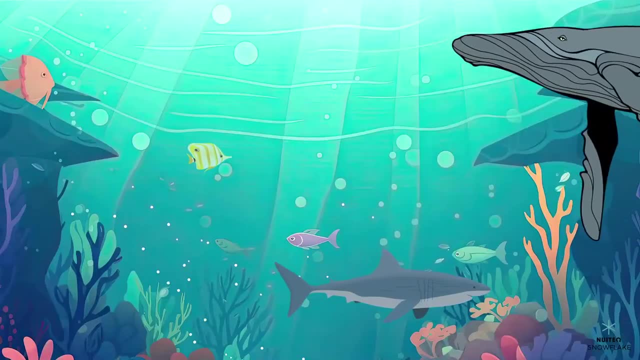 For example, if you go to the jungle, you'll find many different types of animals. You'll find monkeys, birds and snakes, and they are all different from each other. The same thing goes for the ocean: You'll find different types of fish, sharks and whales. 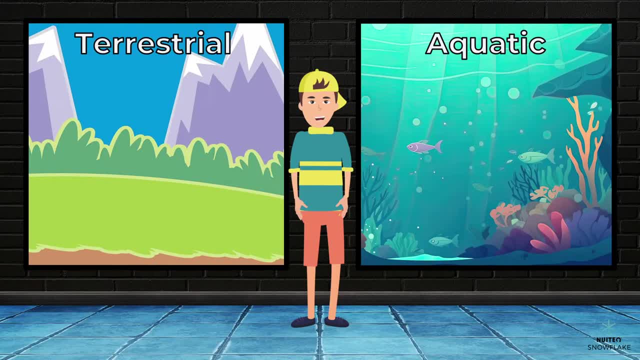 So what's the difference between terrestrial and aquatic animals? Well, terrestrial animals have adapted to live on land. They have legs or wings to move around and they breathe air through their lungs. Aquatic animals, on the other hand, have adapted to live on land. 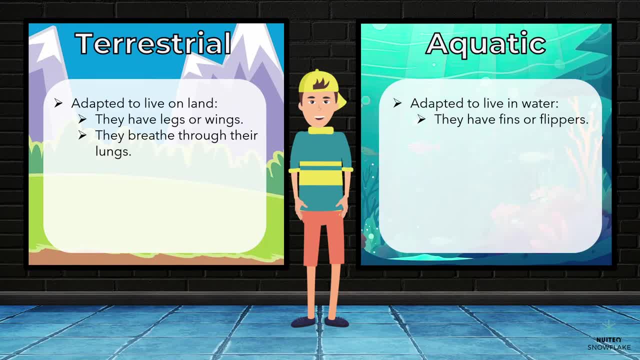 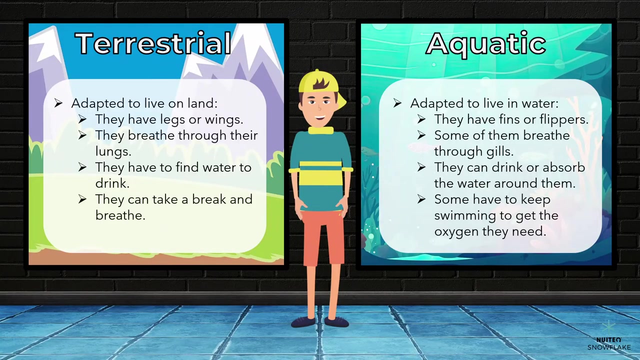 They have fins or flippers to swim, and some of them breathe through gills. Terrestrial animals also have to find water to drink, while aquatic animals can just drink or absorb the water around them. Some aquatic animals, like fish, have to constantly swim to get the oxygen they need to survive, while terrestrial animals can take a break and just breathe. 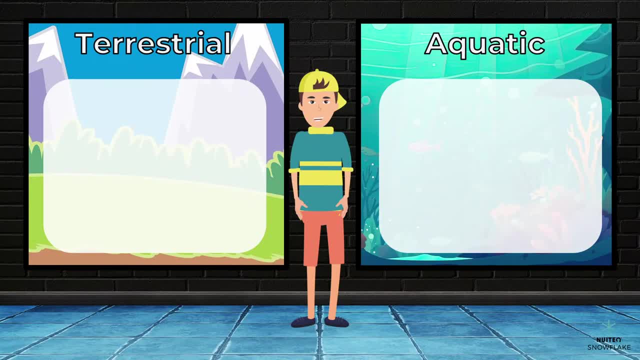 In terms of diversity, there are many different types of terrestrials. There are terrestrial animals like mammals, birds, reptiles and insects. Aquatic animals also have a lot of diversity, from small creatures like plankton to big ones like whales. 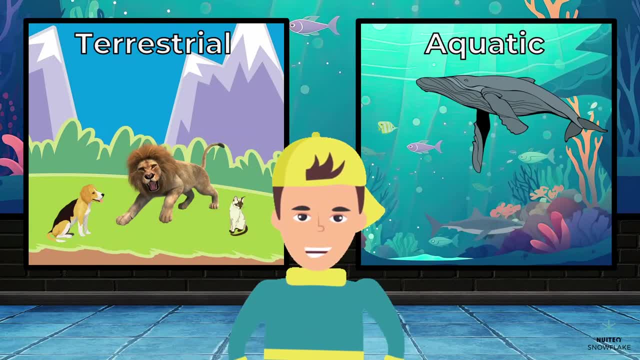 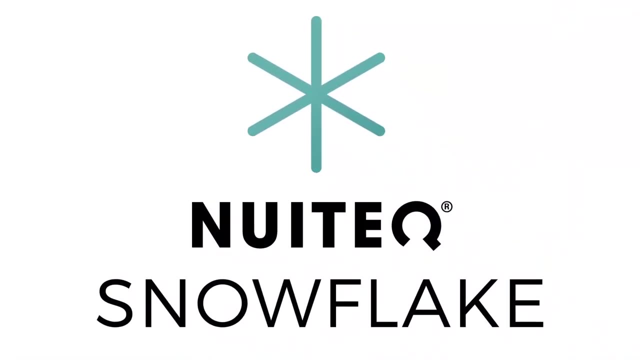 So there you have it. Terrestrial animals live on land, while aquatic animals live in water. They both have different adaptations and are diverse in their own ways. Keep learning and exploring the wonderful world of animals. For more information, visit wwwfemagov.